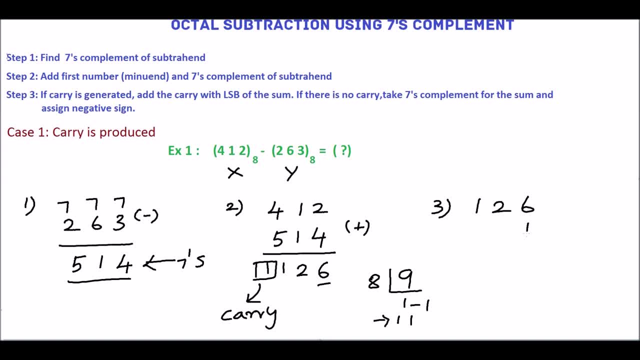 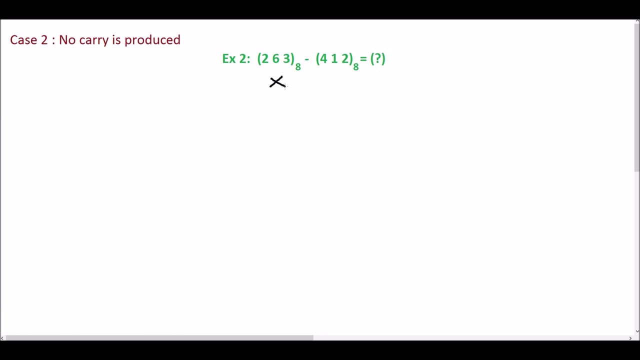 this sum of 126 and the carry end-around, carry 6 plus 1, is 7.. 2 is 1.. The answer is 127, base 8.. Next we will move to the example 2.. We will assign the numbers as x and y. Step 1, find the. 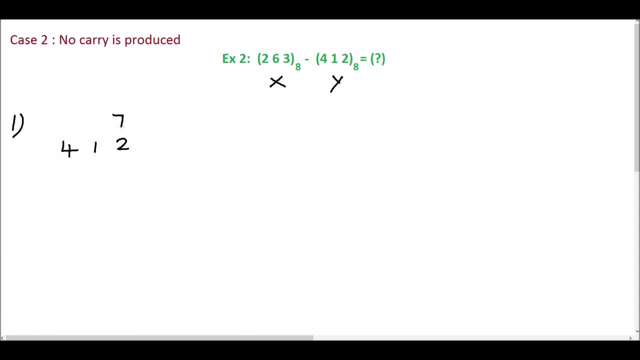 Subtract the digits from number 7, 7-2 is 5,, 7-1 is 6,, 7-4 is 3, which is the 7th complement of y. In step 2, add x and 7th complement of y, which is 3,, 6, 5.. Add this: 3 plus 5. 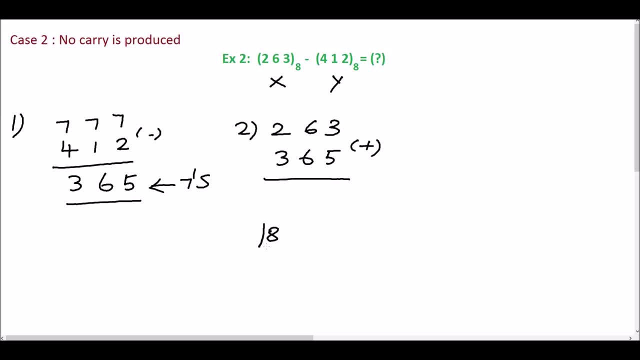 is 8.. 8 is not an octal number. We will convert this 8 into octal. The quotient is 1 and the remainder is 0. So the equivalent octal number is 1, 0.. 0 is the sum and 1 is the. 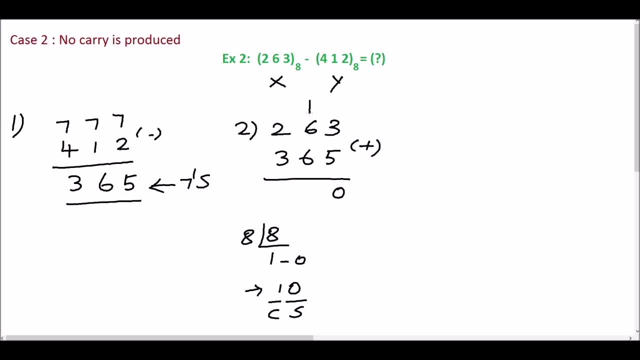 carry. Write sum. carry here: 1 plus 6 plus 6 is 13.. 13, also not an octal number. We will convert this into octal. The quotient is 1 and the remainder is 5.. So 1, 5 is the equivalent. 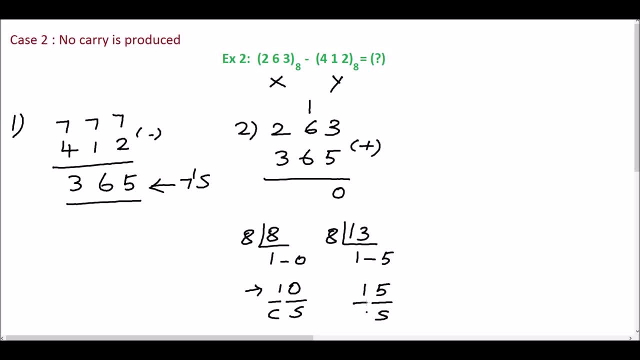 octal. In this 5 is the sum and 1 is the carry. Write 5 here and the carry here. 1 plus 2 plus 3 is 6.. In step 2, the carry is not generated. So take the 7th complement for the sum Sum is 6, 5, 0.. This is the sum. Take 7th complement. 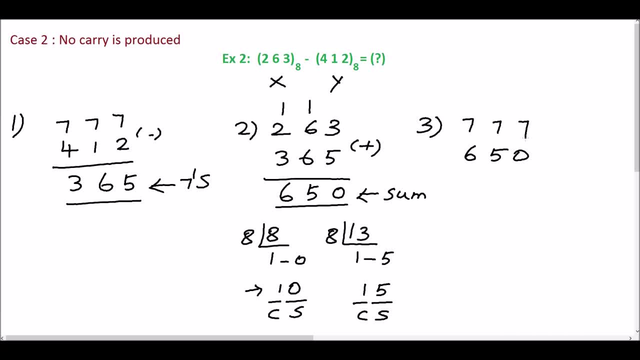 for this, Subtract the digits from 7.. 7-0 is 7, 7-5 is 2, 7-6 is 1.. Finally, assign negative sign to this 7th complement. So the answer is minus 127 base 8.. We will summarize the steps. First, find the 7th complement.